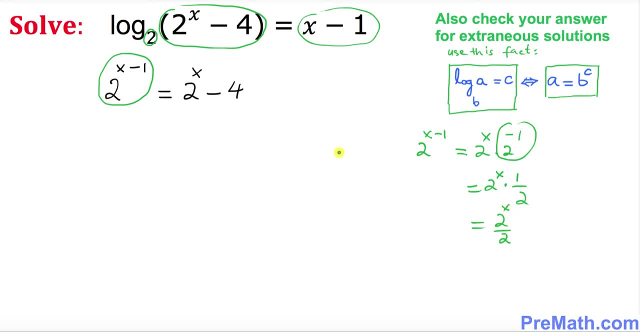 could be written as 2 power x over 2.. So that means I can replace this, whatever this stuff is, by 2 power x divided by 2 equals to 2 power x minus 4.. Now, once again, we want to make this. 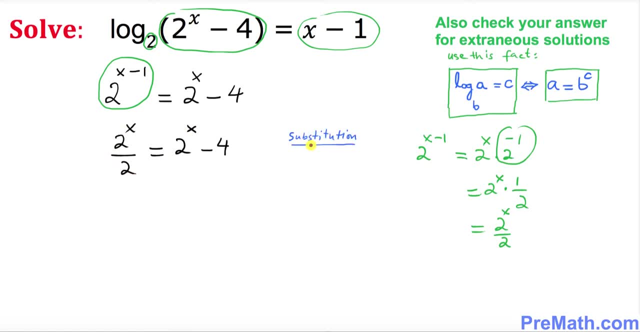 simpler again. So this time we will be using a substitution method. That means, wherever you see 2 power x, I'm going to replace it by u. So I'm going to say: let u equals to 2 power x. So this equation is going to become simply: u over 2, equal to u minus 4.. Now I want to. I can do one thing. 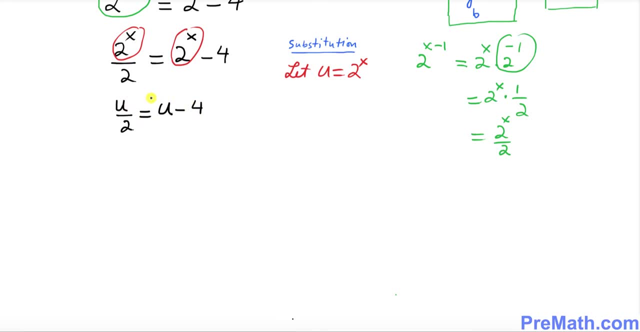 over here. I want you to turn things, switch things around the direction. I want you to put u minus 4 on this side and u over 2 on this side. Does it make any difference? None whatsoever. So I want you to move this 4, negative 4 on this side And, at the same time, I want you to move 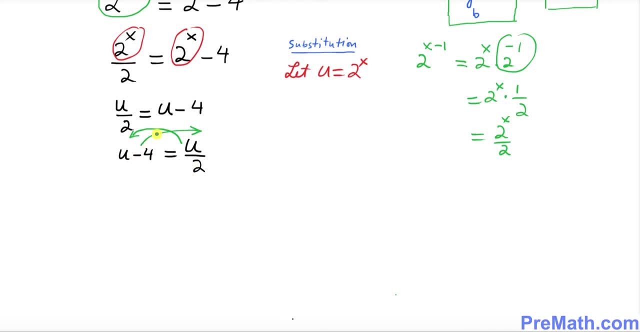 this: u over 2 on the left hand side. So this is what is going to happen: u minus 4 is u? u over 2, when you move it on the other side, become negative: u over 2.. And this negative. 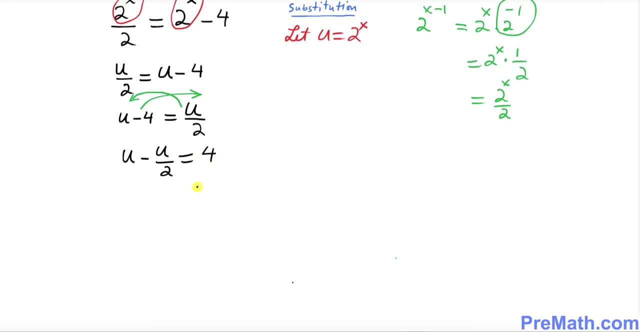 4 becomes positive 4.. Now look at this thing: We have a u and you are taking away half of the u. That means we are ended up with u over 2 equals to 4.. So far, so good. Now we want to get rid of. 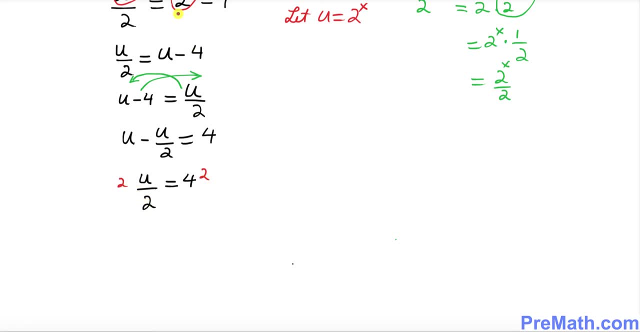 this 2.. We're going to multiply by 2 on both sides. So once you multiply this one, this 2 and 2 is gone. So u turns out to be 2 times 4 is 8.. So u turns out to be 8.. 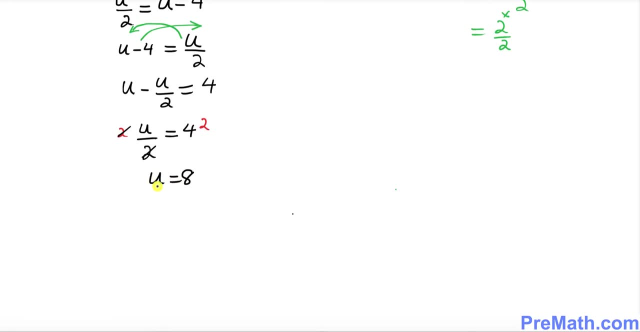 Now the next step is we want to revert it back to a x variable. So, as you recall that u was 2 power x when we did the substitution, So I'm going to replace u by 2 power x, equals to 8.. Now one more thing: 8 could be written as 2 power 3.. As long as these two bases. 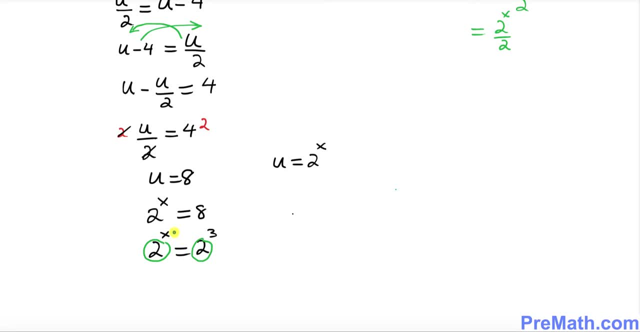 2 and these two are same, that means that this, this, your, you can set these exponent equal to. So that means we can write x equals to 3.. Thus 3 is our. that means it's our solution. So x equals to x is that means x equals to 2 power, x mixed. 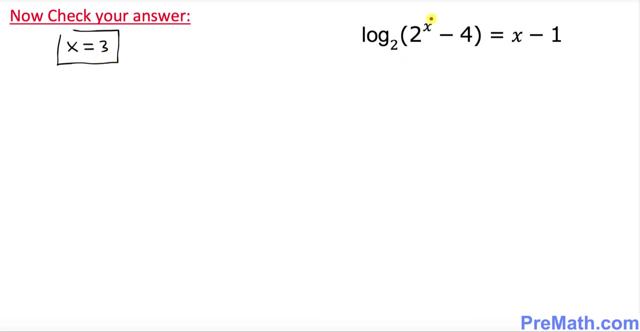 with 9, So x equals to x, is our solutions. and then, finally, what are we going to do now? We're going to find the x, So x equal to 3誕作 3 minus 4. with a base, 2 equals to where X is again 3 minus 1. let's see what. 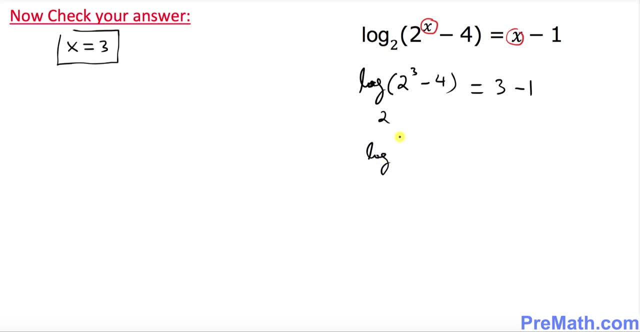 happens. so log of 2- power 3 is 8 minus 4- with a base 2 turns out to be equal to 2, are simply log of 4 with a base 2 equals to 2. so far, so good. and now, once again. 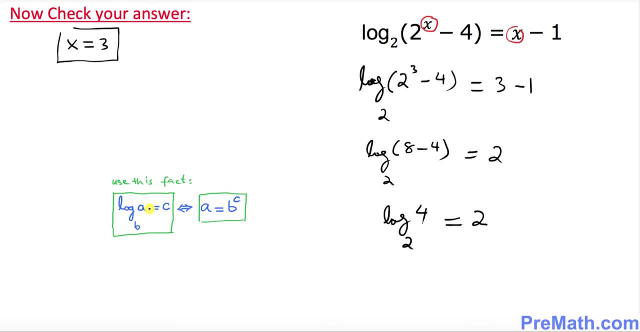 we will be using this fact. if we want to convert from logarithmic form to exponential form, we can write as this: one 4 equals to 2 power 2, so 4 equals to 4.. isn't it two? power two is only the base two. as a base one plus man, the base one minus two of x 2 equals to: 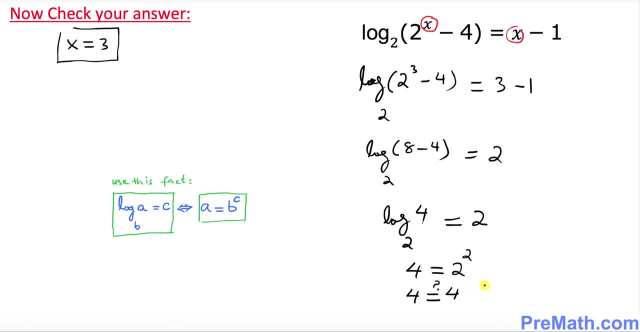 4.. Now my question is: is this a true statement? Yes, this is a true statement. Thus, x equal to 3 is indeed our solution. Thanks for watching and please subscribe to my channel for more exciting videos.